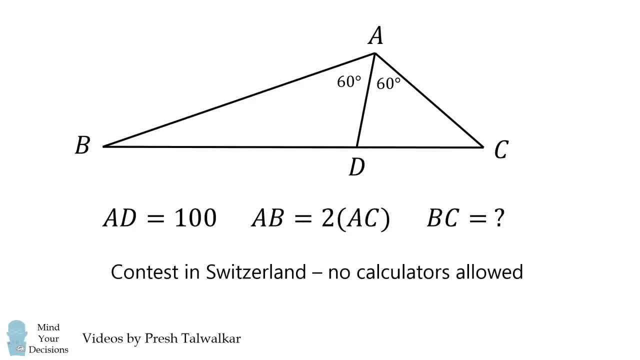 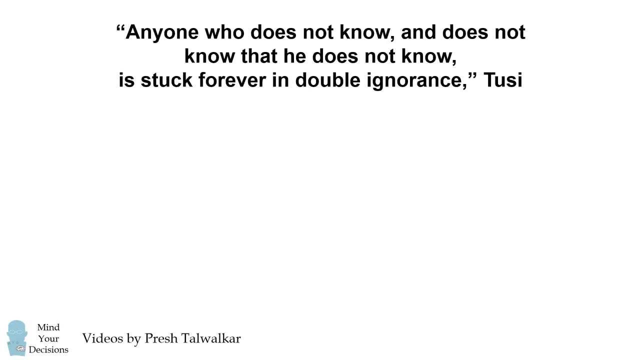 This was asked in a math contest in Switzerland and no calculators were allowed. Pause the video if you'd like to give it a try and, when you're ready, keep watching to learn how to solve this problem. So let's get started solving this problem. 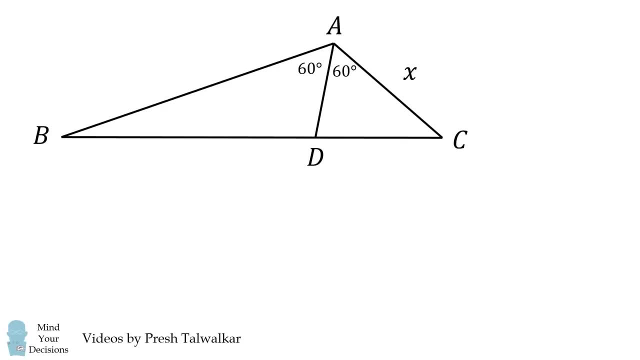 If AC has a length of X, then AB is equal to 2X. Now we are going to solve this problem. We are going to prove that BD is equal to 2 times DC. This follows immediately by the angle bisector theorem. 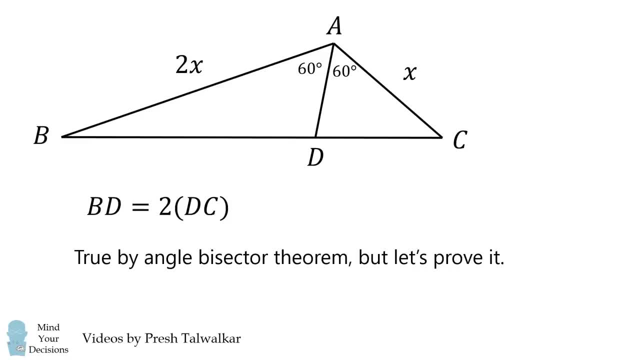 but if you didn't remember the angle bisector theorem, let's prove it. So let's get started by labeling angle ADC as alpha. Then angle ADB will be supplementary, so it will be 180 degrees minus alpha. Next we'll use the law of sines, which I read was first described by the Persian mathematician Tusi. 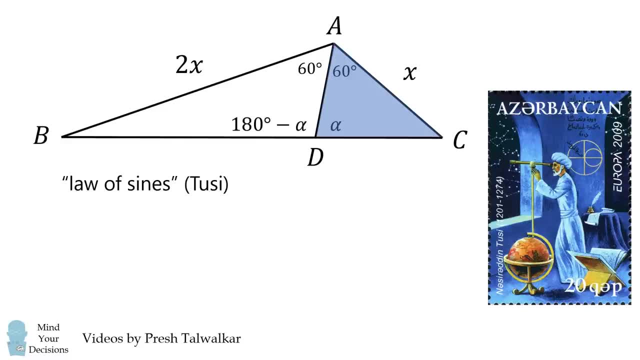 So let's use the law of sines in triangle ADC. This gives that DC divided by the sine of 60 degrees is equal to X divided by the sine of alpha. Next, we'll use the law of sines in triangle ADB. 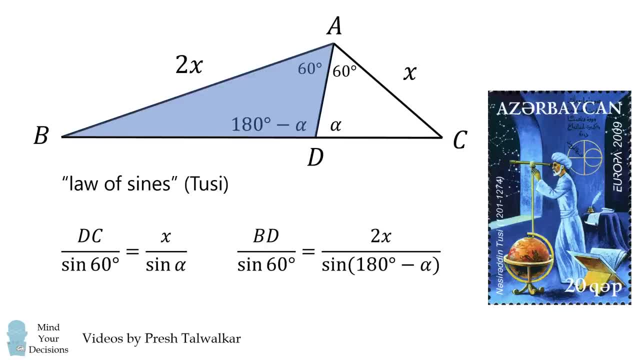 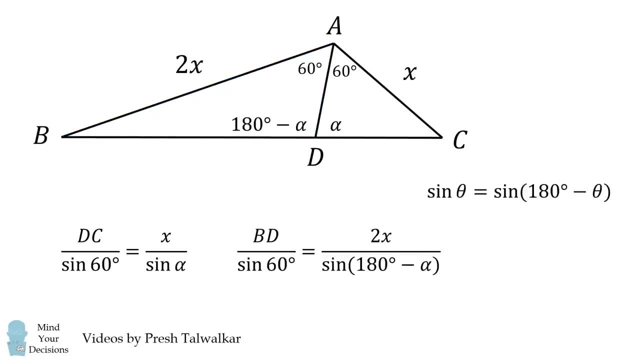 This gives that BD divided by the sine of 60 degrees is equal to 2X divided by the sine of the angle, 180 degrees minus alpha. Next, we use the identity that the sine of an angle is the same as the angle bisector theorem. 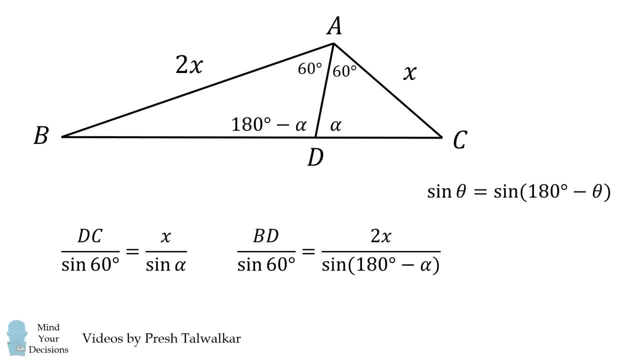 This gives that BD divided by the sine of 60 degrees is equal to 2X divided by the sine of the angle 180 degrees minus alpha as its supplementary angle. so we can simplify this fraction. Now let's multiply both equations by the sine of 60 degrees. 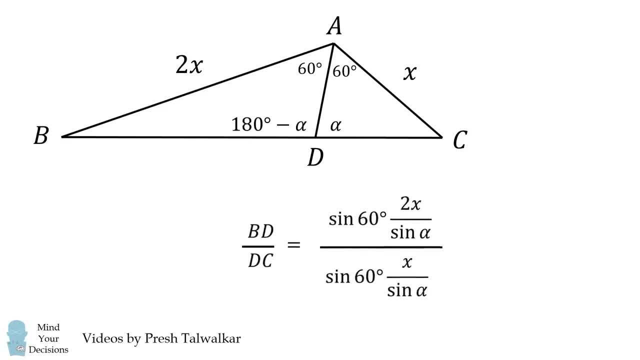 and then we'll divide the first equation from the second equation, We get the ratio BD to DC. We can now cancel out many terms. We're left with just the fraction equal to 2, and this will directly lead to the identity that we want. BD is equal to 2 times DC. 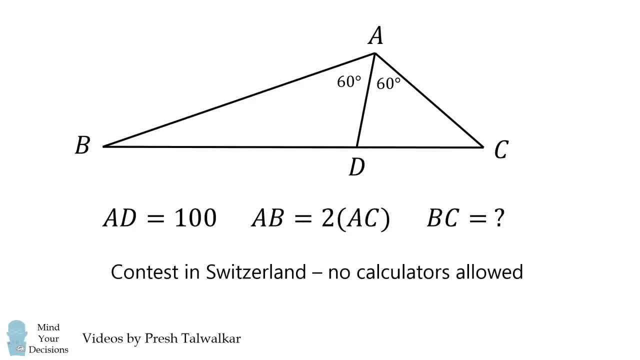 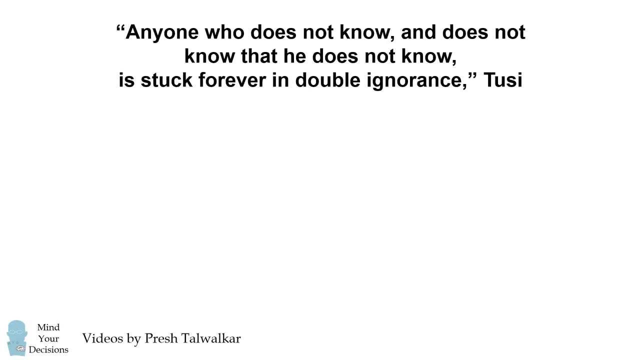 This was asked in a math contest in Switzerland and no calculators were allowed. Pause the video if you'd like to give it a try and, when you're ready, keep watching to learn how to solve this problem. So let's get started solving this problem. 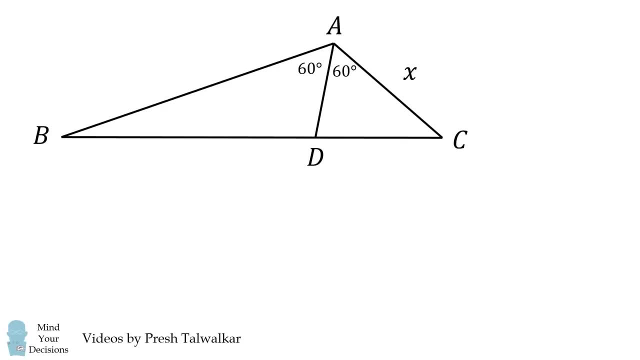 If AC has a length of X, then AB is equal to 2X. Now we are going to solve this problem. We are going to prove that BD is equal to 2 times DC. This follows immediately by the angle bisector theorem. 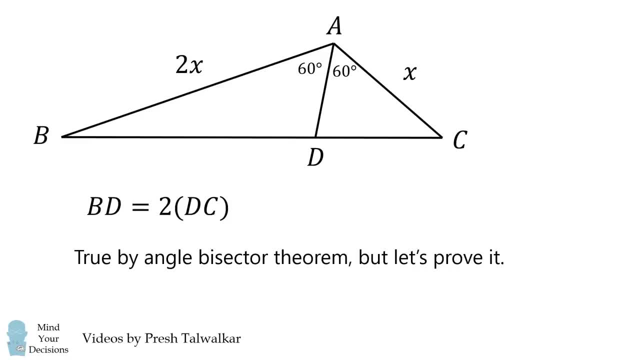 but if you didn't remember the angle bisector theorem, let's prove it. So let's get started by labeling angle ADC as alpha. Then angle ADB will be supplementary, so it will be 180 degrees minus alpha. Next we'll use the law of sines, which I read was first described by the Persian mathematician Tusi. 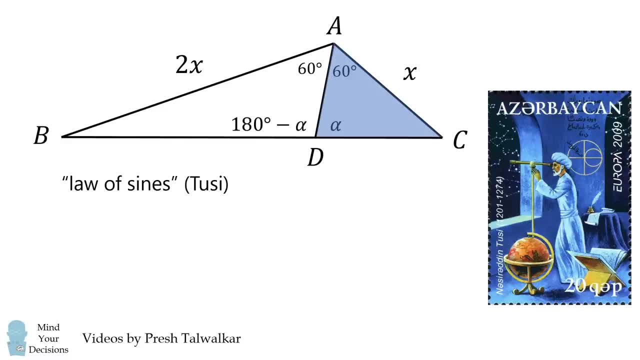 So let's use the law of sines in triangle ADC. This gives that DC divided by the sine of 60 degrees is equal to X divided by the sine of alpha. Next, we'll use the law of sines in triangle ADB. 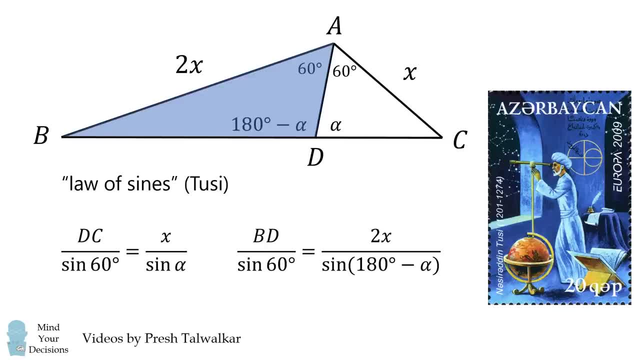 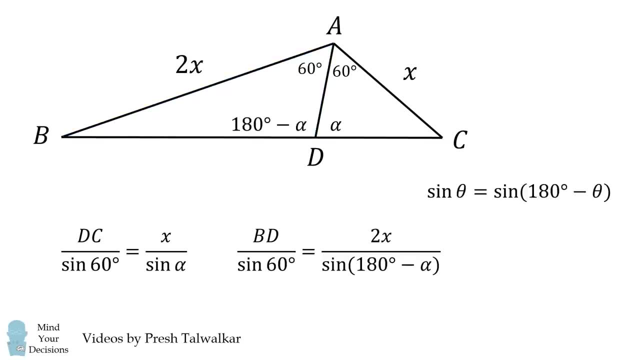 This gives that BD divided by the sine of 60 degrees is equal to 2X divided by the sine of the angle, 180 degrees minus alpha. Next, we use the identity that the sine of an angle is the same as the angle bisector theorem. 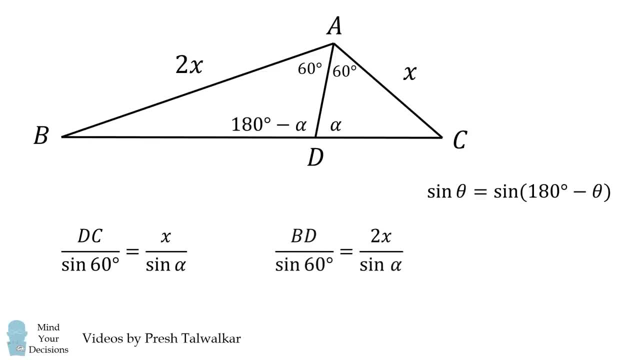 as its supplementary angle. so we can simplify this fraction. Now let's multiply both equations by the sine of 60 degrees and then we'll divide the first equation from the second equation. We get the ratio BD to DC. We can now cancel out many terms. 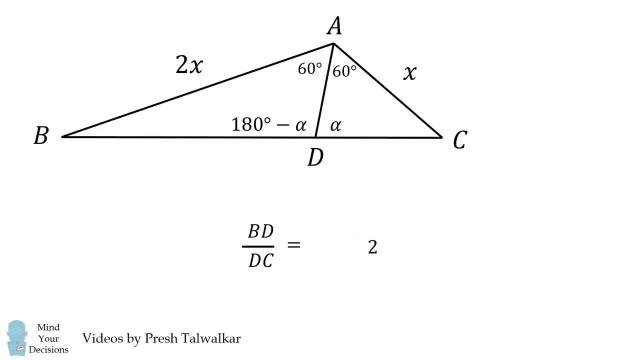 We're left with just the fraction equal to 2, and this will directly lead to the identity that we want. BD is equal to 2 times DC, So if DC has a length of Y, BD will have a length of 2Y. 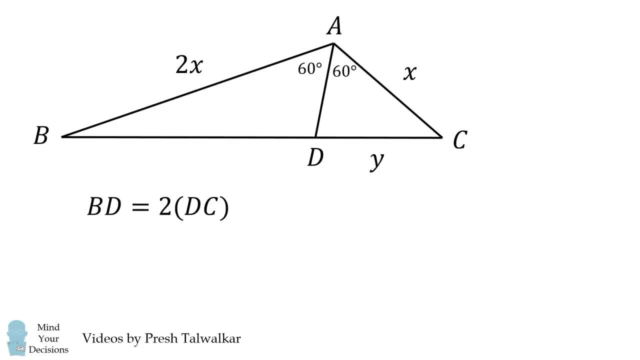 So if DC has a length of Y, BD will have a length of 2Y. Now recall that the length of AD is 100.. Now we're going to use Alkashi's theorem: Y squared will be equal to X squared plus 100 squared minus 2 times X, times 100, times the cosine of 60 degrees. 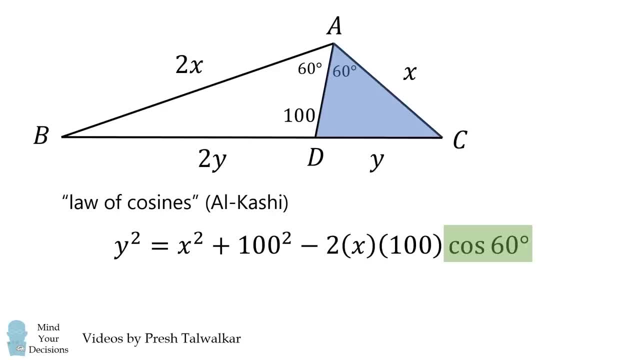 Since the cosine of 60 degrees is equal to 1 half, we'll simplify this. We'll put this equation to the side and now we'll use Alkashi's theorem on this triangle. We again simplify the cosine of 60 degrees and we get this equation. 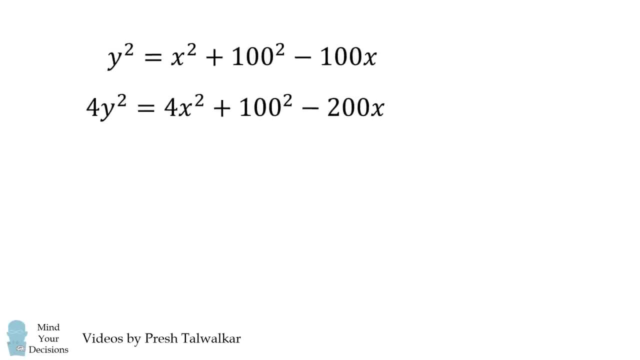 So we now have two equations. Let's cancel out the Y squared terms. We'll multiply the first equation by 4, and then we'll subtract the second equation. We'll cancel terms between the equations And we're left with: 0 is equal to 3 times 100 squared minus 200 X. 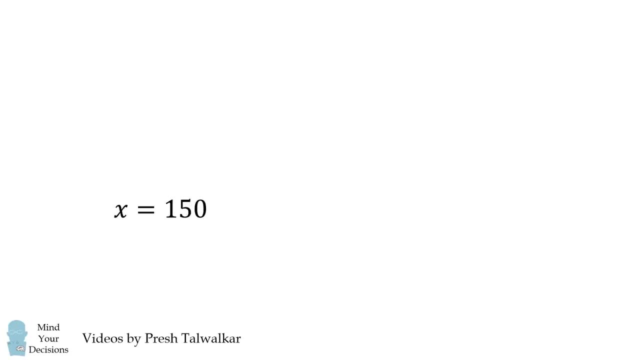 We can then solve that X is equal to 150.. We then go back to our diagram and then we're going to use the law of cosines or Alkashi's theorem and we're going to substitute in for X. We get that Y squared is equal to. 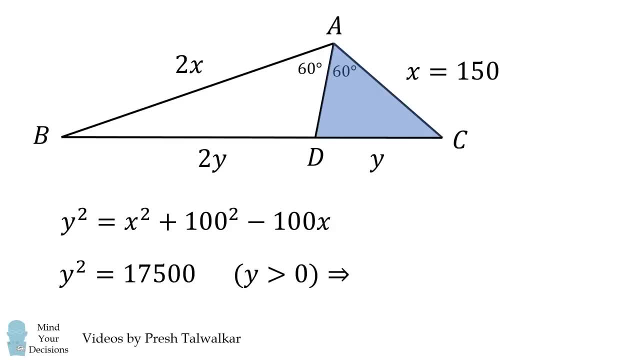 17,500, and then that means Y. we want to take the positive value because we're dealing with a length. Y will be equal to 50 times the square root of 7.. Now recall: we want to solve for BC, and BC is equal to 3Y, so we get 150 times the square root of 7.. 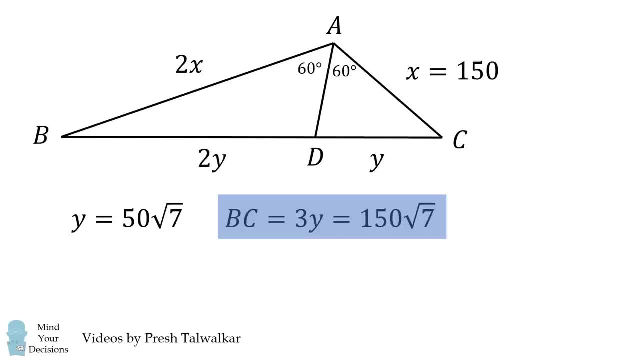 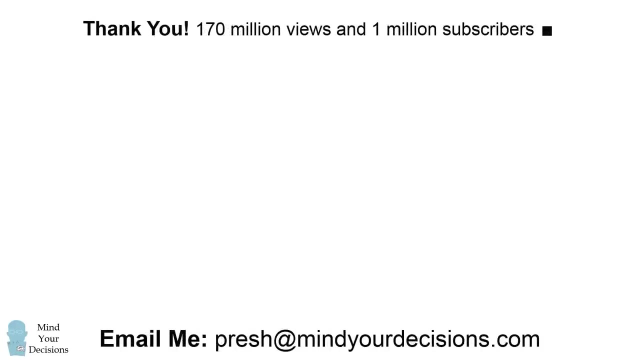 And that's our answer. So I think this is a great trigonometry problem, because you really have to use a lot of concepts to work out the final answer, And you can do it all without a calculator. Thanks for watching and for making Mind Your Decisions. one of the best channels on YouTube. 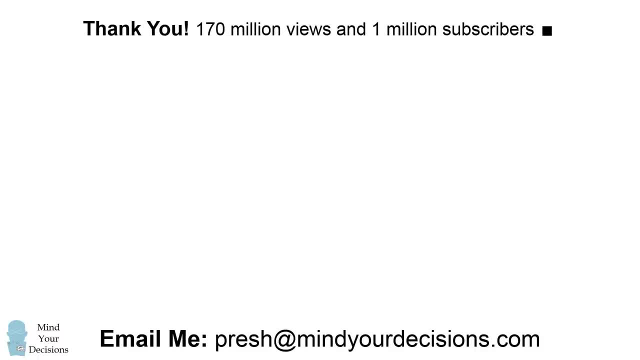 Thanks for watching and thanks for your support. Subtitles by the Amaraorg community.